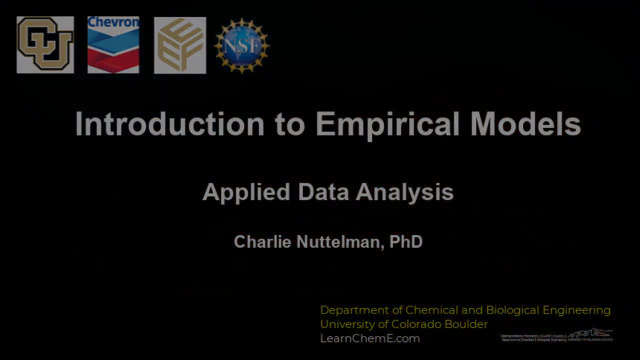 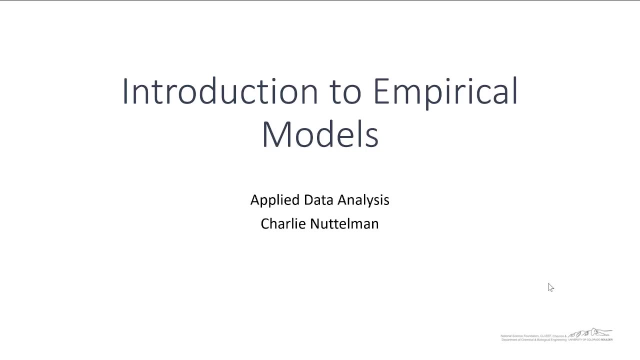 In the next couple of weeks we're going to be talking about empirical models, mathematical modeling and regression models, And so I'm just going to kind of give you an introduction to empirical models. in this screencast, Natural phenomena is described by some process We have 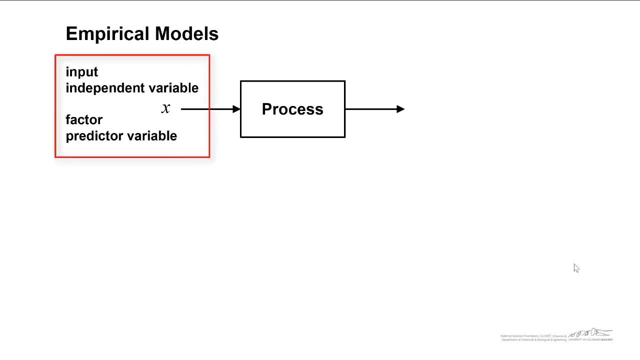 an input. This is also known as an independent variable or a factor or a predictor variable. This goes into some sort of process, whether that's a natural process or a synthetic or a chemical process, some sort of chemical reaction or mechanical process- And we have an output- This 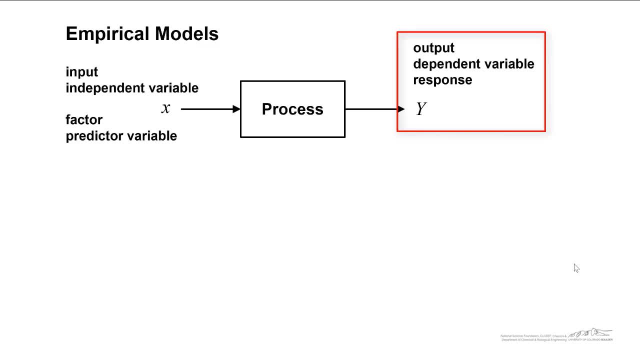 is known as the dependent variable. It depends upon the independent variable. Oftentimes we will refer to this as the response, And our job as engineers and scientists is to try to model this process. We try to put together some, something that we can use to model the process, And we try to model the process And we try to 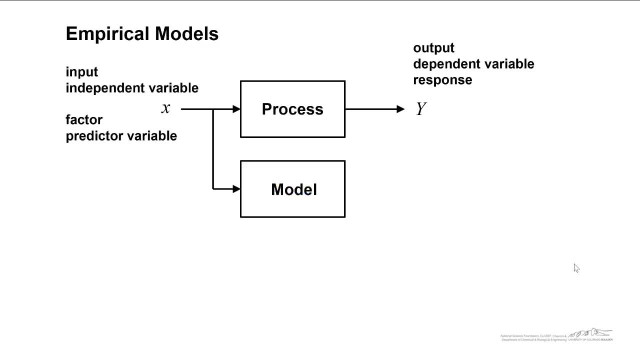 sort of mathematical model where we take into account the independent variable- There could be multiple independent variables going into this, by the way- And we try to come up with a prediction. This hat above the y represents the prediction or the estimate, And ideally we would create this. 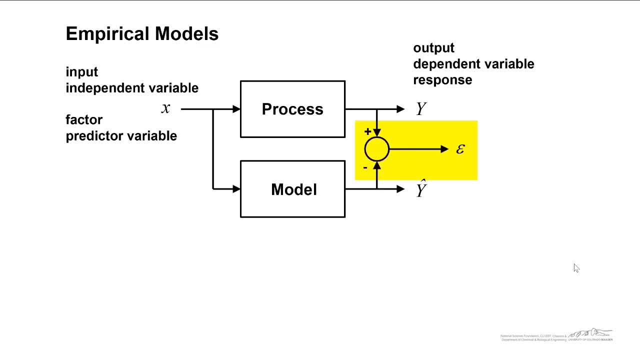 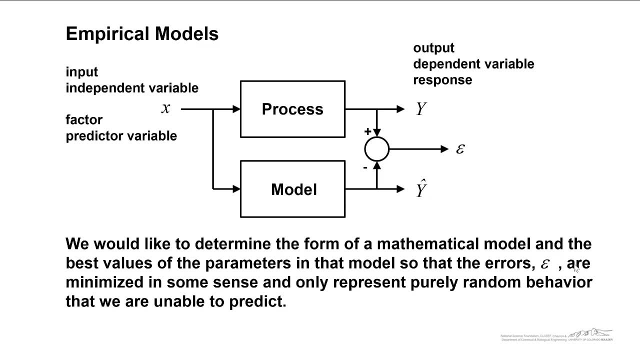 model such that the only difference between the model prediction and the actual output is just random error denoted by this epsilon. We would like to determine the form of a mathematical model and the best values of the parameters in that model, so that the errors are minimized in some. 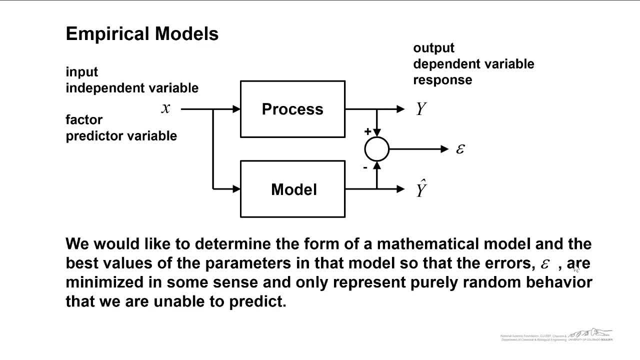 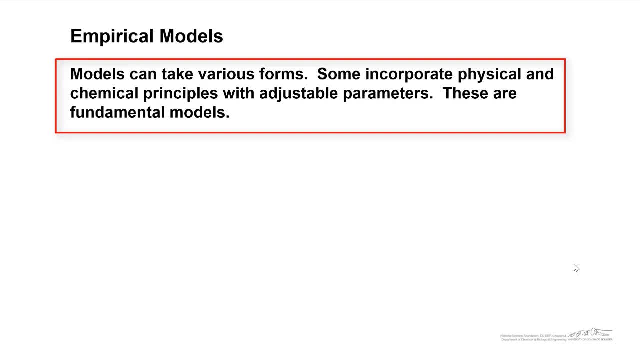 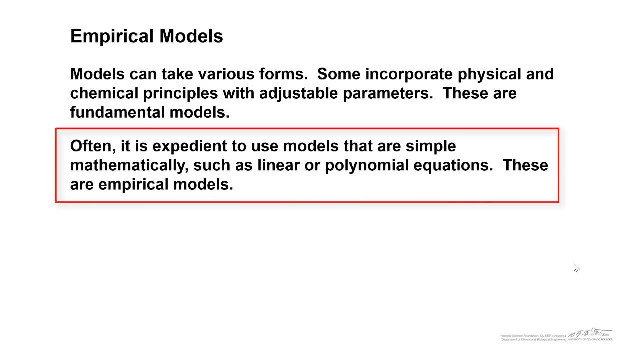 sense and only represent purely random behavior that we are unable to predict. Models can take various forms. Some incorporate physical and chemical principles with adjustable parameters. These are known as fundamental models. Often it is expedient to use models that are simple mathematically, like linear or polynomial equations, And these are empirical models, Occasionally models. 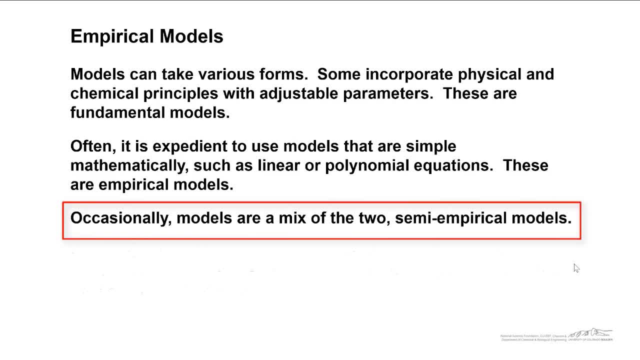 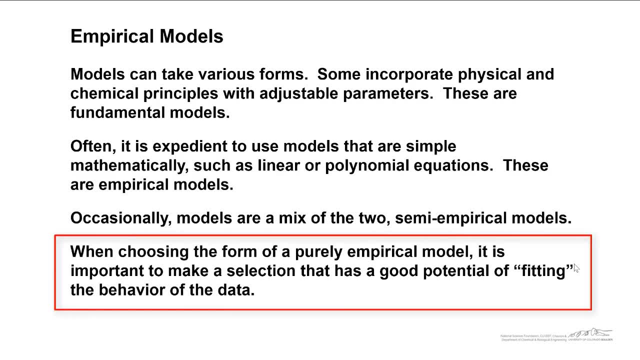 are a mix of the two, And these are known as semi-empirical models. When choosing the form of a purely empirical model, it is important to make a selection that has a good potential of fitting the behavior of the data. The first step in choosing an empirical model is to look at the 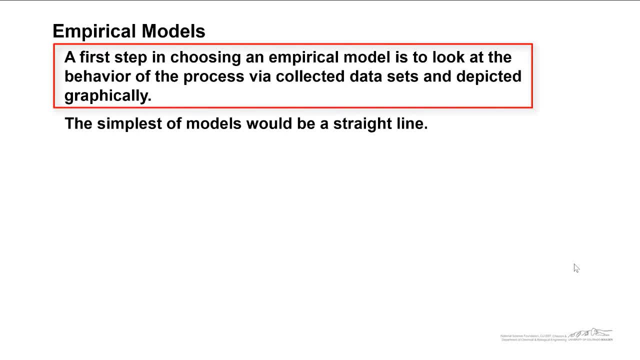 behavior of the process via collected data sets and depicted graphically. The simplest of models is a straight line And many of you have seen the equation for this before. Our model prediction is some function of the behavior of the data And we want to know the behavior of the data And we 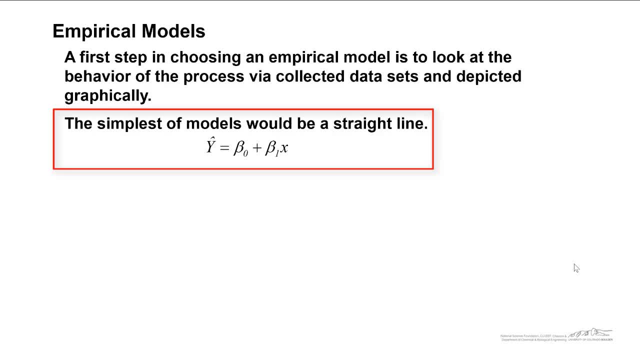 want to know the behavior of the data And we want to know the behavior of direct change. The attribute price is a function of the data We can calculate. what does this mean in terms of the correlation of check? and this refers to the zoals Kirkland, than hemos pleased to represent how the value of a general f brutal. 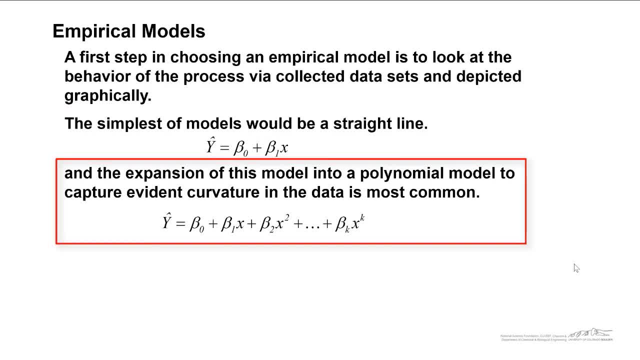 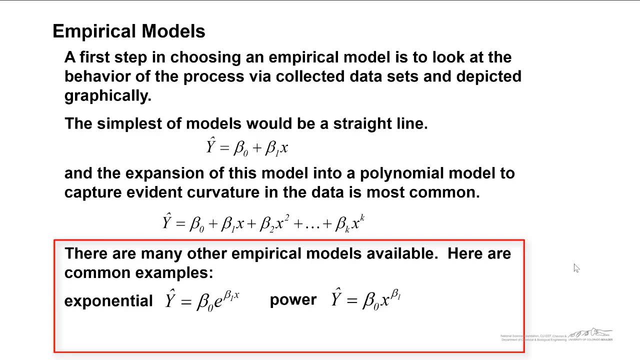 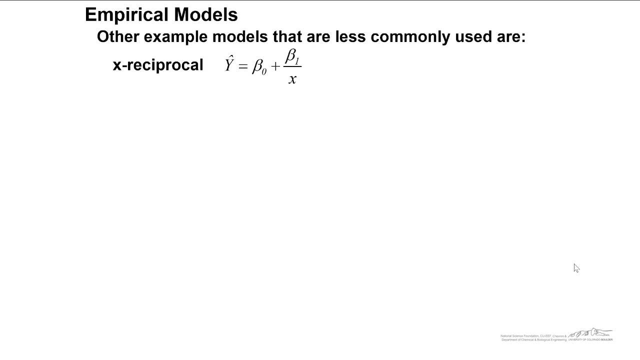 occurred and of an V1, of an intercept beta-naught and a slope beta-one, And the expansion of this model depends on. based on a各位 you have used models, We have an x. reciprocal y equals beta naught plus beta 1 over x, We have a y. 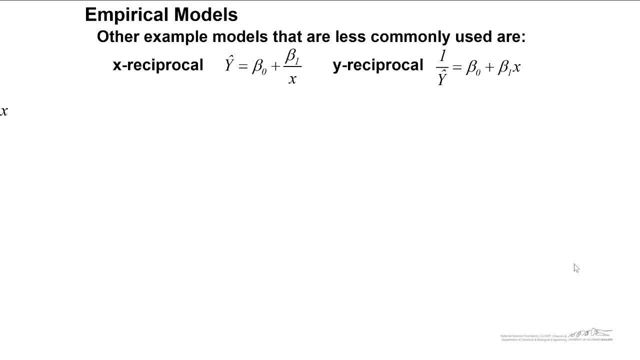 reciprocal 1 over y. hat is beta naught plus beta 1- x, We have an xy ratio, an x exponential. So there's lots of different candidate models that you can look into. The appropriate way to know whether one of these models is a candidate is to observe its behavior for different parameter. 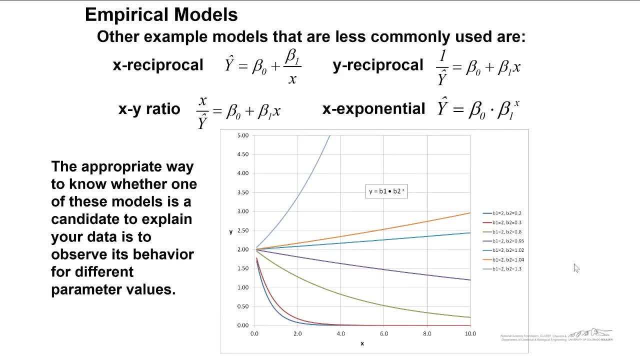 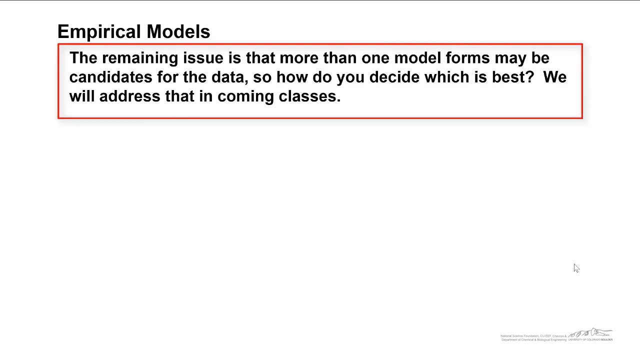 values. Here we have an x exponential model and depending upon the different parameters- b1 and b2, you can see that it can change quite dramatically. The remaining issue is that more than one model forms may be candidates for the data. so how do you decide which is best? You? 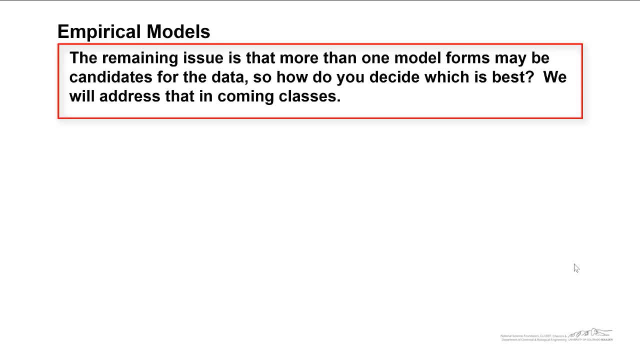 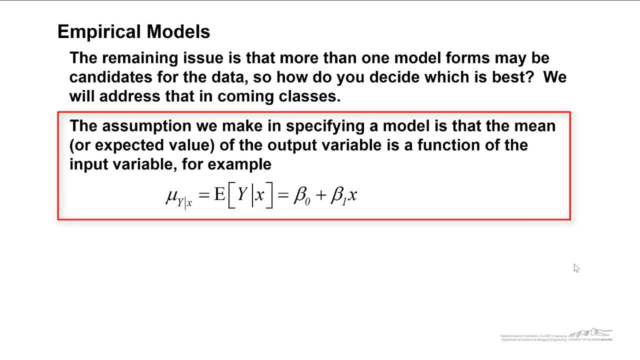 guys are going to learn in this class how to choose which model is the best for the data among several candidates. The assumption we make in specifying a model is that the mean, also known as the expectation value, of the output variable- so that's mu y- is a function of the input variable. The mean of the 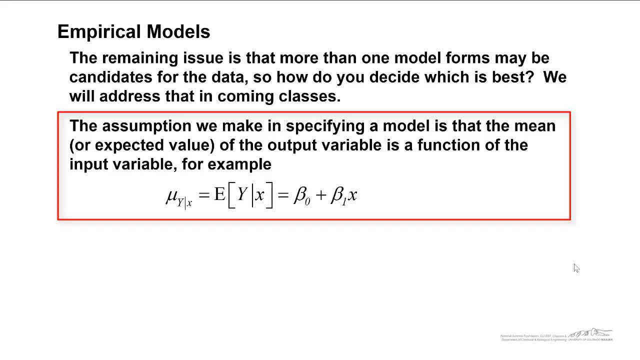 output at any value of x is simply beta naught plus beta 1 x. That doesn't mean every time you put in the same value of x you're going to get the same output. but if you were to look at the probability density function, it's going to be normally distributed about some value That depends upon.